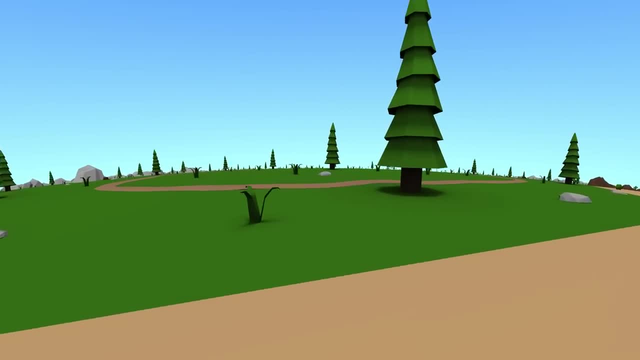 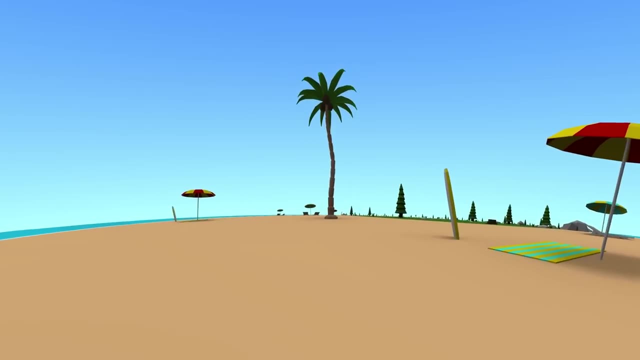 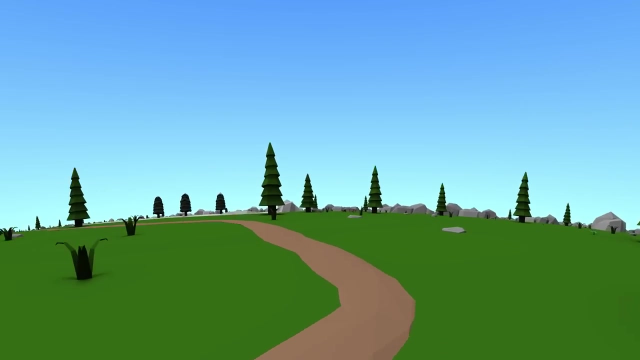 it's quite the opposite. In general, hyperbolic geometry looks like a more exaggerated Euclidean geometry. You know, because it's hyperbolic, Things appear to get smaller, faster. more space fits into the same perceived space. but things seem, overall, familiar. But let's 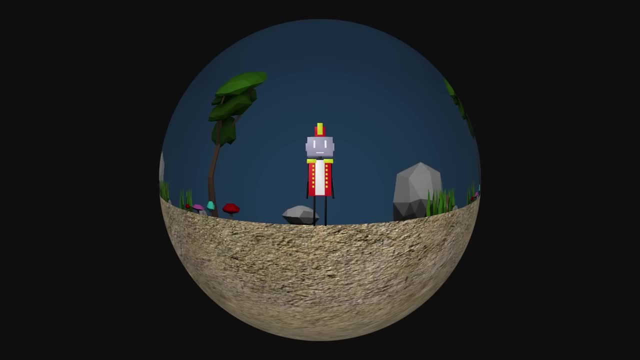 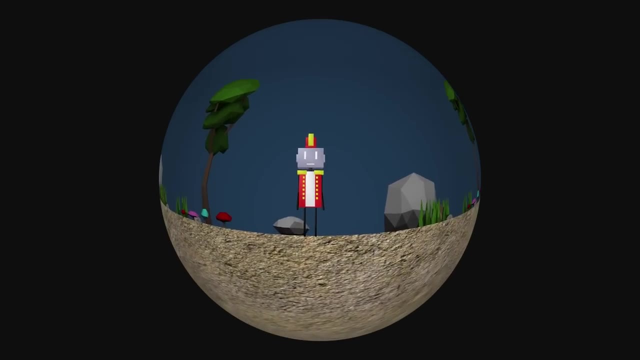 take a trip to spherical flatland. We'll just say that everything below the equator is underground and everything above is open space, So we can jump up and down and walk around. In fact, if we keep walking in either direction, we'll eventually come back to 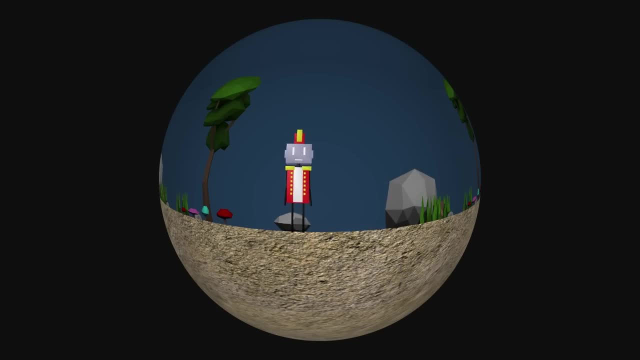 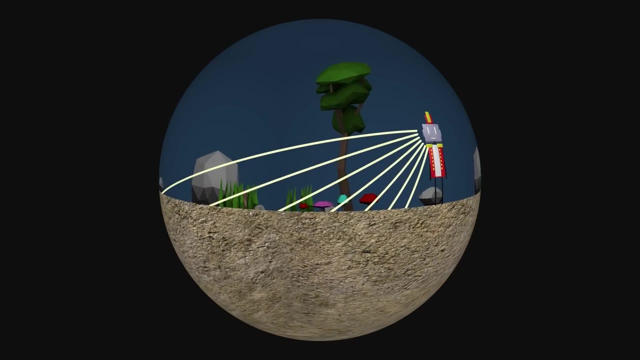 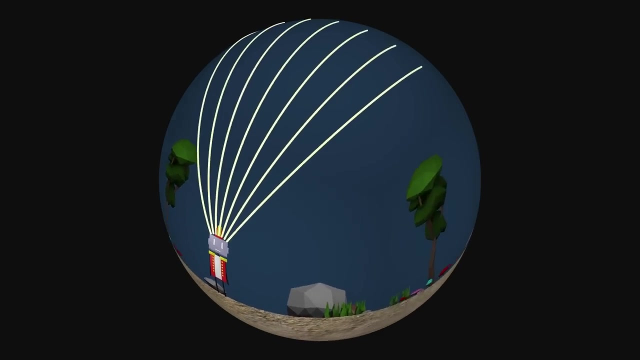 where we started, But what would you actually see? Let's cast some rays from our perspective to see what happens. Objects close by aren't really affected much and look like you'd expect, But an object on the other side- Well, look how many of our light rays hit this rock, This tiny object. 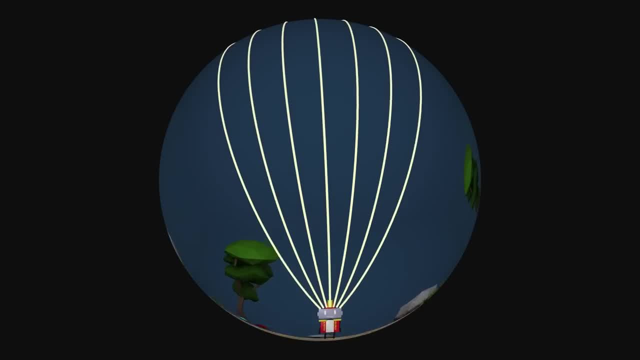 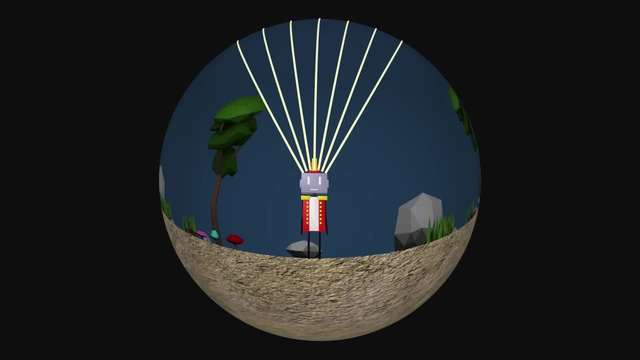 literally on the other side of the world, would look enormous in the sky and appear upside down, Sort of like a giant magnifying lens. The result is a reverse perspective. Farther away objects can appear larger than closer to the ground. Also, notice that all rays eventually hit the ground. There's no sky per se, at least not. 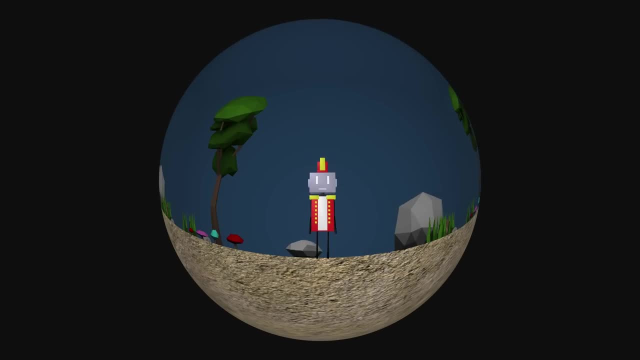 one you can see without using fog or a draw distance. Alright, are you ready to go up one dimension higher? We're going to switch to first person now, but all the same things I just talked about in 2D apply to 3D. 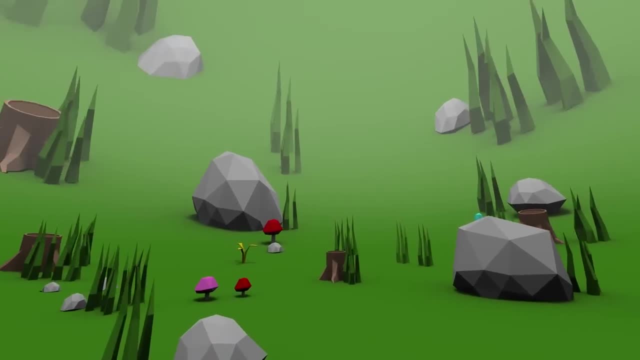 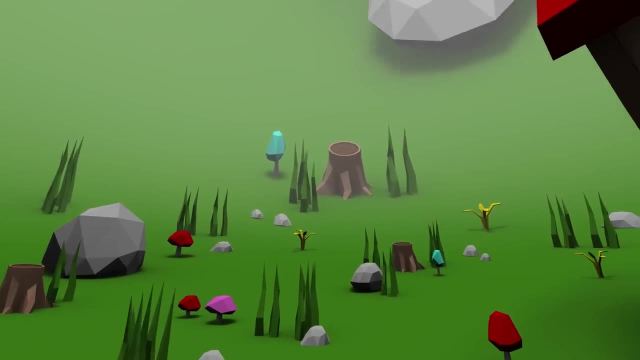 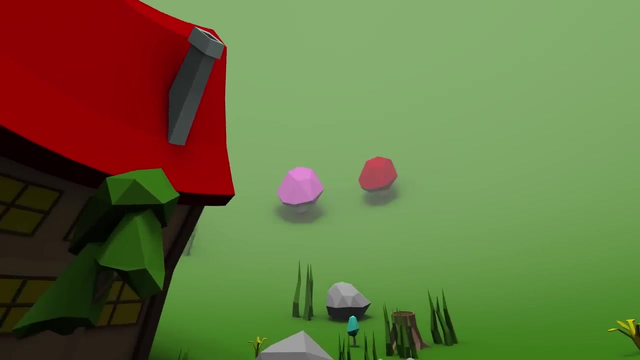 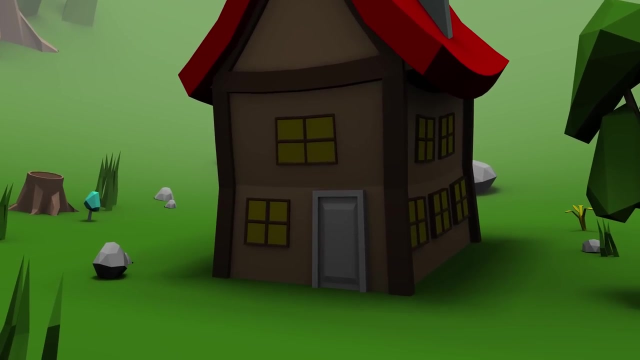 It should be pretty obvious now why I chose the title of this video. The reverse perspective is obvious. far away, things appear huge and flipped upside down. Take a look at this house. It's pretty normal up close. But now let's go to the opposite.